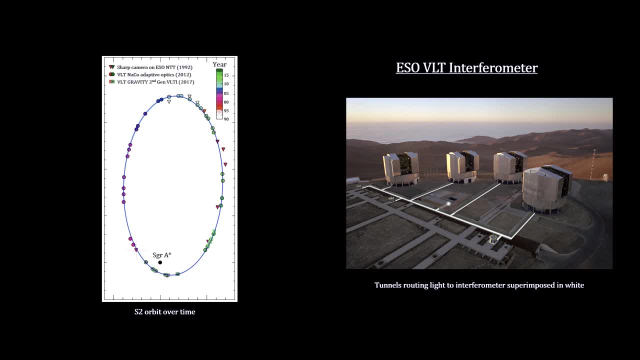 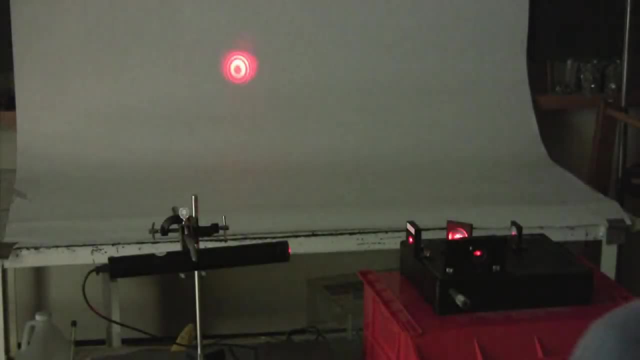 They can even resolve sunspots on nearby stars. So to understand how we know how close S2 got to Sag A star, we need to understand how these stellar interferometer telescopes work. In the Speed of Light chapter of the How Far Away Is It? video book. 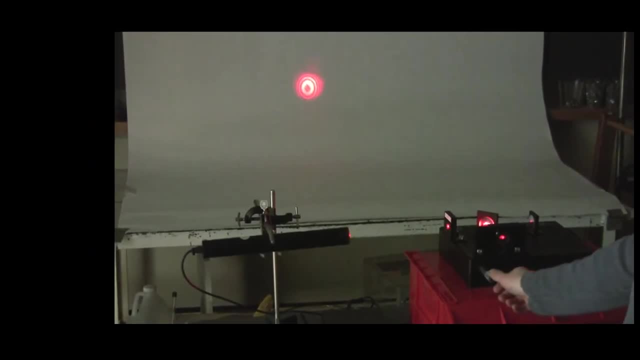 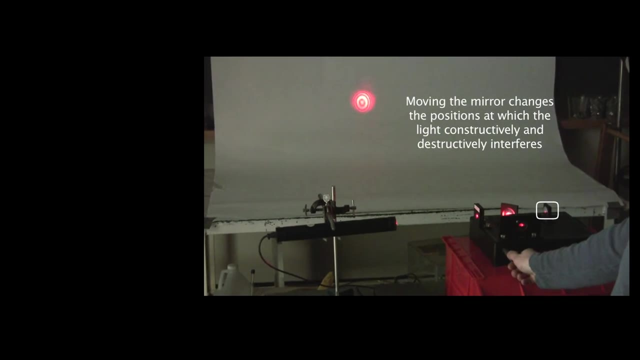 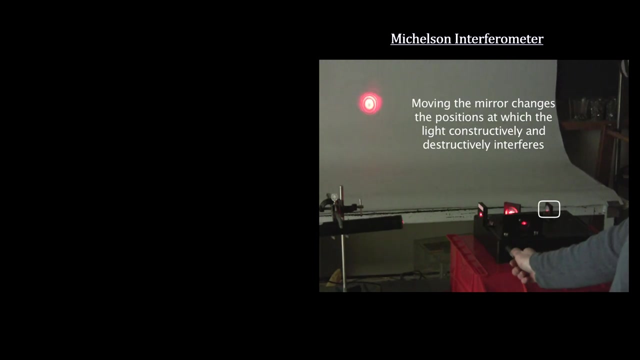 we covered. the Michelson interferometer used to measure minute distances in the lab. Interferometers can measure distances on the order of a few nanometers. Michelson and Morley used it to show that the speed of light was a constant. In order to create light interference, Michelson illuminated the interferometer with fully coherent light. 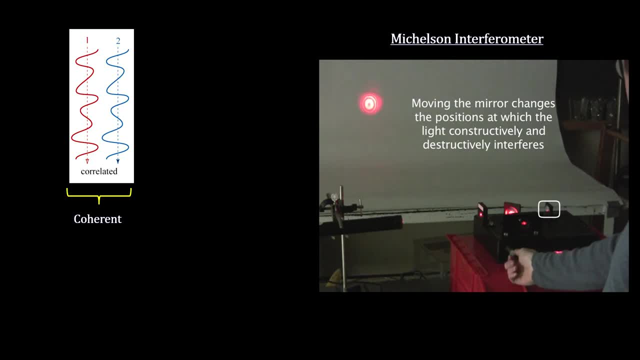 Coherent light has a common frequency and phase. It always produces interference patterns. on the far side of a double slit, Fully coherent light, like the kind that lasers create, will produce regions of fully destructive interference, That is, the dark regions have no light falling on them at all. 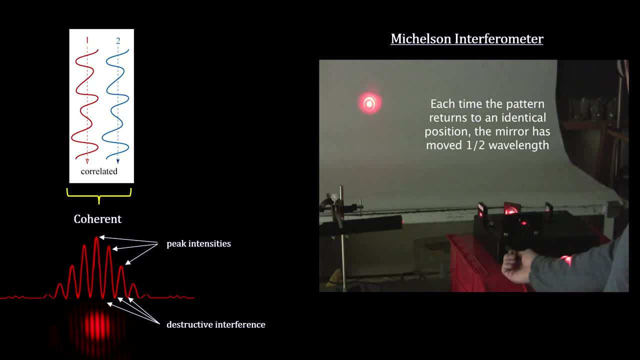 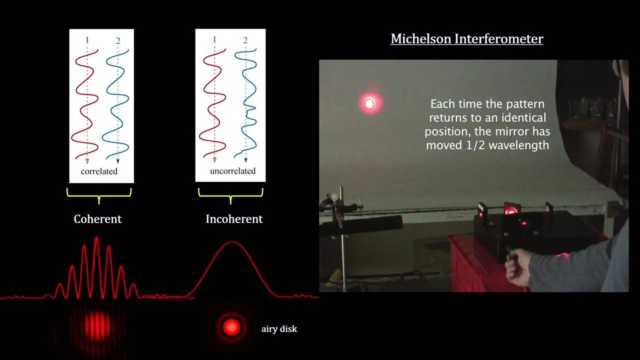 Partially coherent light will produce regions of partially destructive interference, meaning some light falls in the dark regions And incoherent light will not produce interference patterns at all. We find in nature that waves can start out as incoherent and become partially coherent as they spread out. 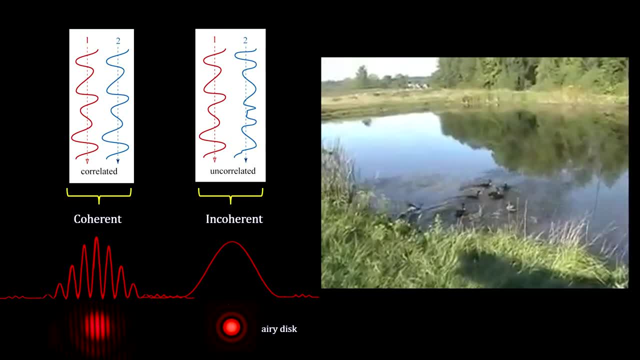 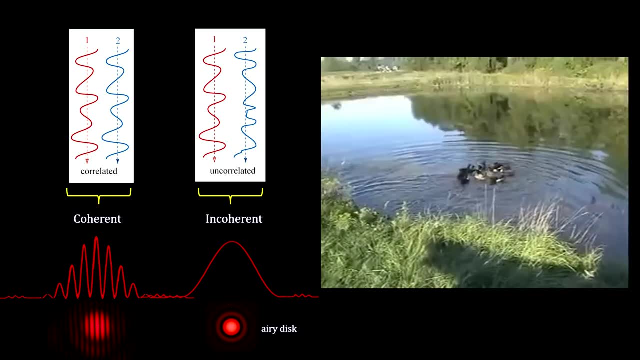 Watch how these ducks start with a chaotic mix of water waves as they enter the pond. Watch how these ducks start with a chaotic mix of water waves as they enter the pond, But as the waves move out they become quite orderly. This is a geometrical effect. 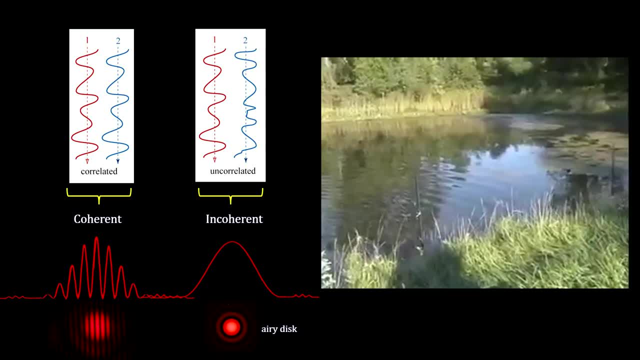 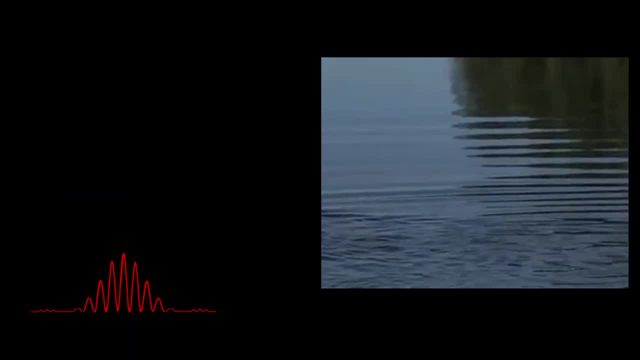 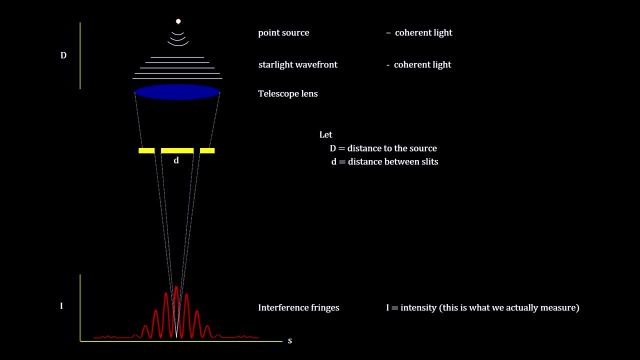 The further away one travels from the source, the less significant the distance between the individual wave generators becomes. A point source for starlight would produce coherent light and at any distance from the source the light would create interference patterns. But there are no point sources in nature. 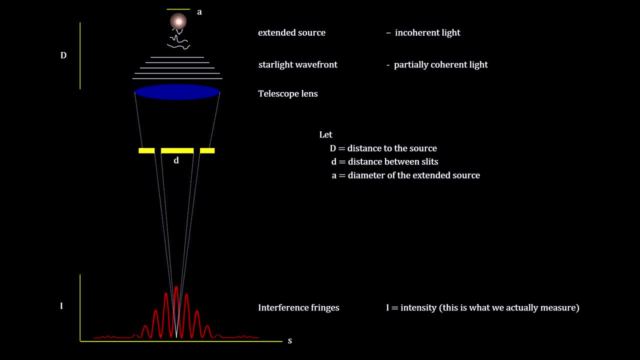 Stars have a diameter on the sky. An extended thermal light source would start out with incoherent light, But as the light moves away from the source its coherence increases, just like with the ducks on the pond: The relationship between the diameter of the source,